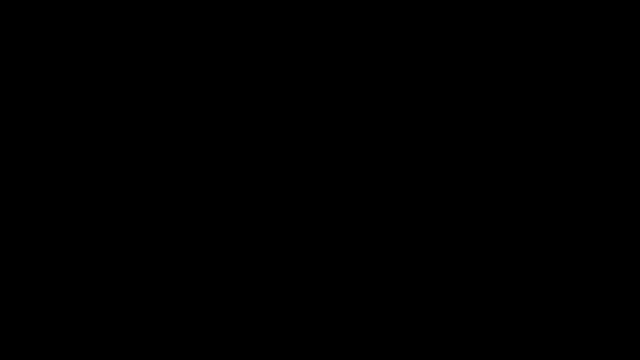 Let's explore a few more methods for solving systems of equations. Let's say: I have the equation 3x plus 4y is equal to 2.5.. And I have another equation: 5x minus 4y is equal to 25.5.. 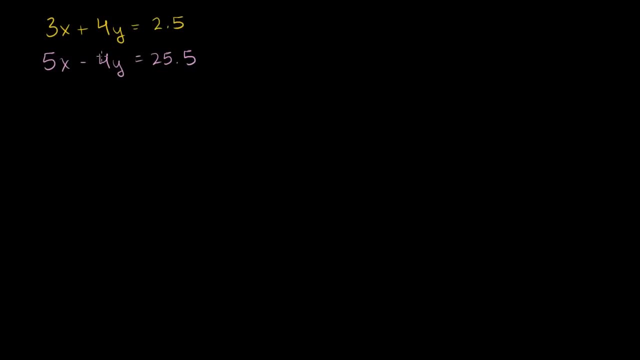 And we want to find an x and y value that satisfies both of these equations. Think of it graphically: This would be the intersection of the lines that represent the solution sets to both of these equations. So how can we proceed? When we saw in substitution, we like to eliminate one of the 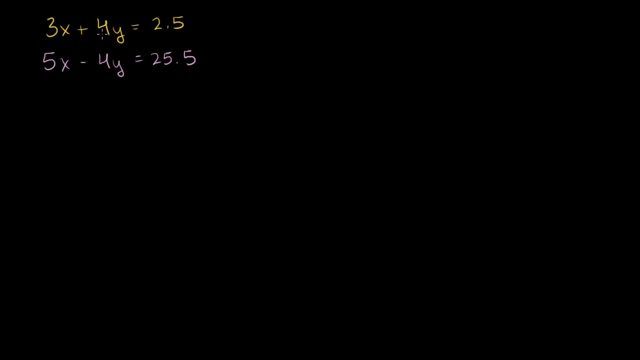 variables. We did it through substitution last time, But is there anything we can add or subtract? Let's focus on this yellow, on this top equation, right here. Is there anything that we can add or subtract to both sides of this equation? Remember, any time you deal with an equation, you have to. 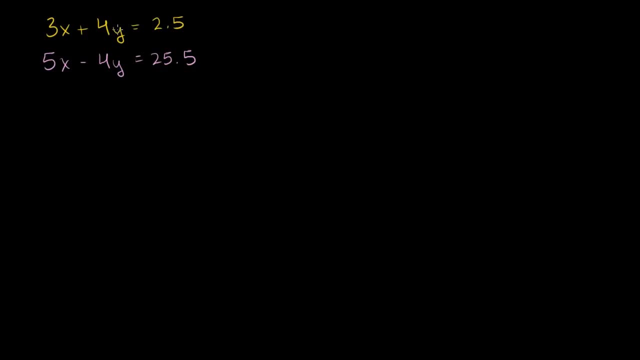 add or subtract the same thing to both sides, But is there anything that we could add or subtract to both sides of this equation that might eliminate one of the variables? And then we would have one equation in one variable and we can solve for it. 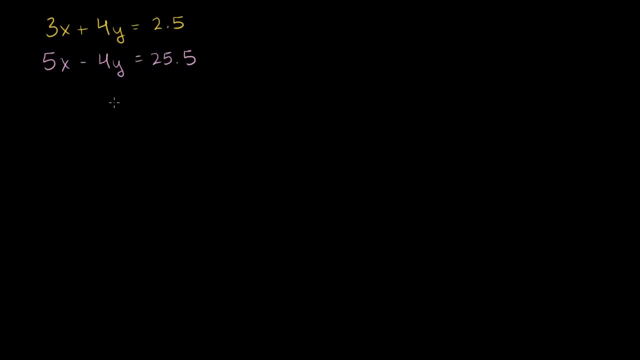 And it's probably not obvious, even though it's sitting right in front of your face. Well, what if we just added this equation to that equation? What I mean by that is what if we were to add 5x minus 4y to 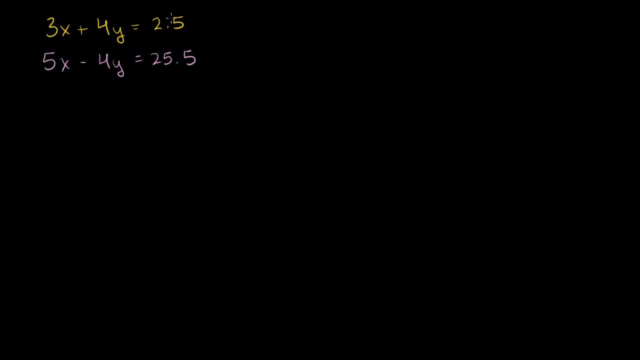 the left-hand side and add 25.5 to the right-hand side. So if I were to literally add this to the left-hand side, I'd add this to the left-hand side and add that to the right-hand side and you're probably saying, Sal, hold on. 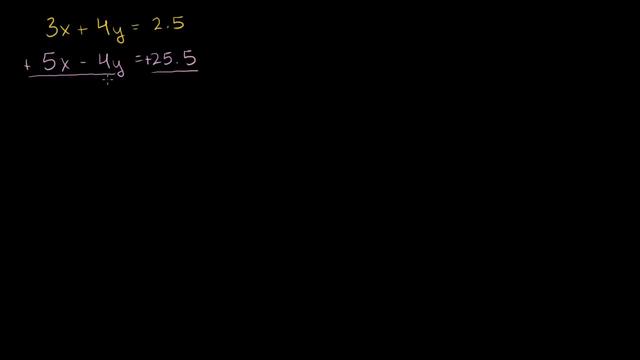 how can you just add two equations like that And remember when you're doing any equation? if I have any equation of the form- well, really any equation- ax plus by is equal to c. if I want to do something to this equation, 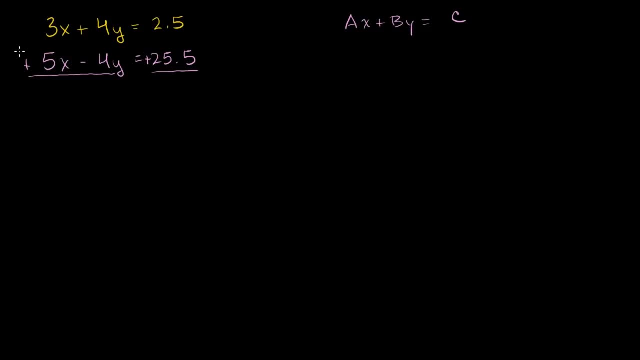 I just have to add the same thing to both sides of the equation. So I could, for example, I could- add d to both sides of this equation- sides of the equation- because d is equal to d, So I won't be changing the equation. 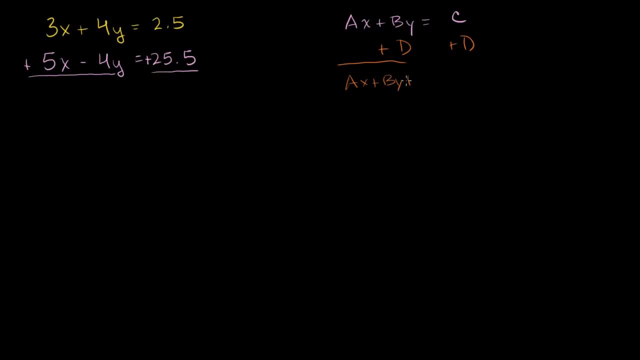 You would get ax plus by plus d is equal to c plus d And we've seen that multiple, multiple times. You can add anything you do to one side of the equation, you have to do to the other side, But you're saying, hey, Sal, wait. 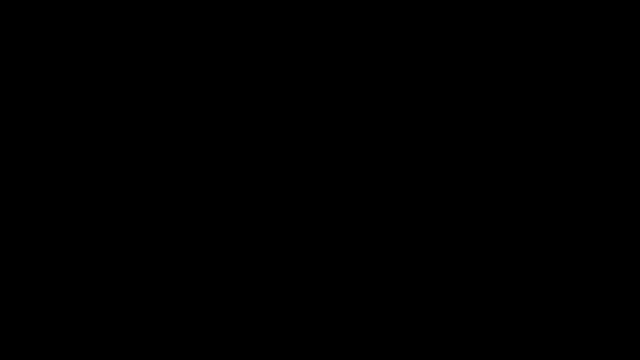 Let's explore a few more methods for solving systems of equations. Let's say: I have the equation 3x plus 4y is equal to 2.5.. And I have another equation: 5x minus 4y is equal to 25.5.. 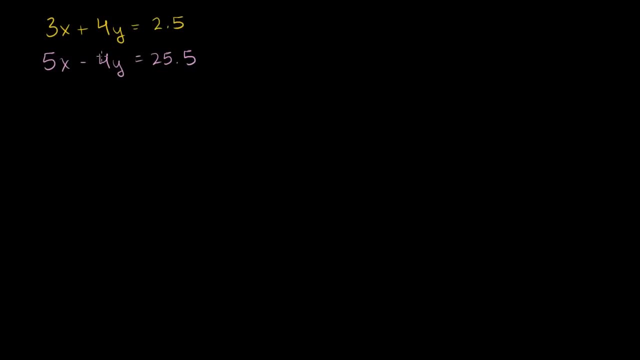 And we want to find an x and y value that satisfies both of these equations. Think of it graphically: This would be the intersection of the lines that represent the solution sets to both of these equations. So how can we proceed? When we saw in substitution, we like to eliminate one of the 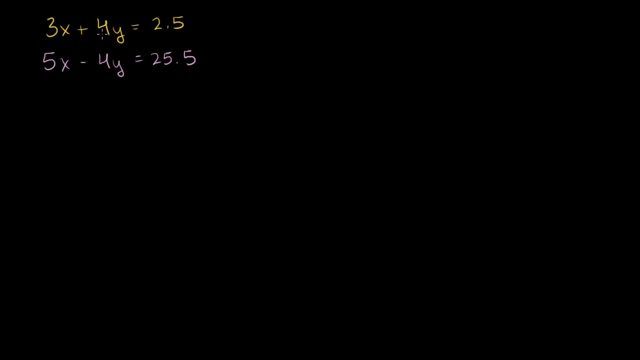 variables. We did it through substitution last time, But is there anything we can add or subtract? Let's focus on this yellow, on this top equation, right here. Is there anything that we can add or subtract to both sides of this equation? Remember, any time you deal with an equation, you have to. 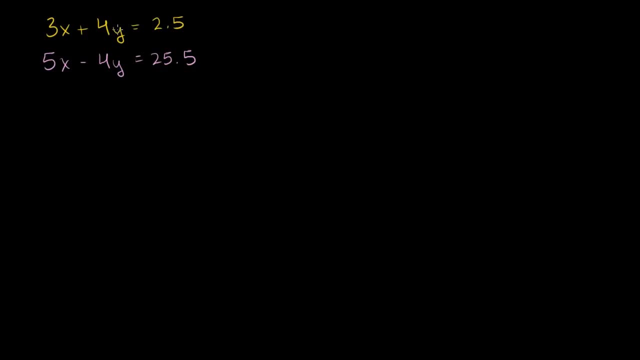 add or subtract the same thing to both sides, But is there anything that we could add or subtract to both sides of this equation that might eliminate one of the variables? And then we would have one equation in one variable and we can solve for it. 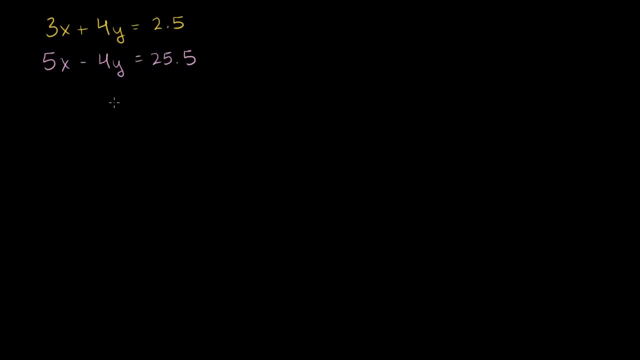 And it's probably not obvious, even though it's sitting right in front of your face. Well, what if we just added this equation to that equation? What I mean by that is what if we would add 5x minus 4y to 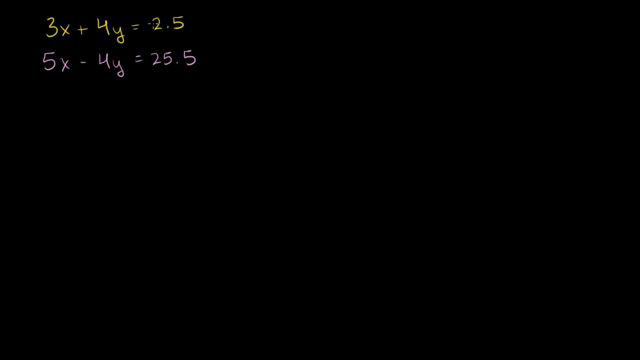 the left-hand side and add 25.5 to the right-hand side. So if I were to literally add this, this to the left-hand side and add that to the right-hand side, And you're probably saying, Sal, hold on. 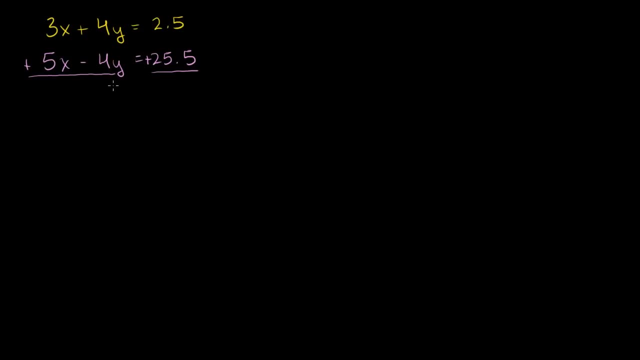 How can you just add two equations like that And remember when you're doing any equation? if I have any equation of the form, well, really any equation- ax plus by is equal to c. if I want to do something to this, 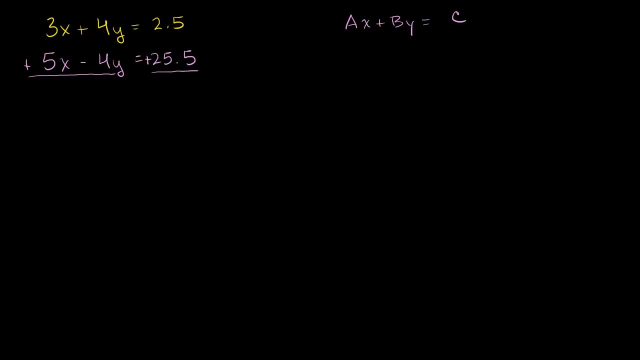 equation. I just have to add the same thing to both sides of the equation, So I could, for example, I could- add d to both sides of the equation because d is equal to d, So I won't be changing the equation. 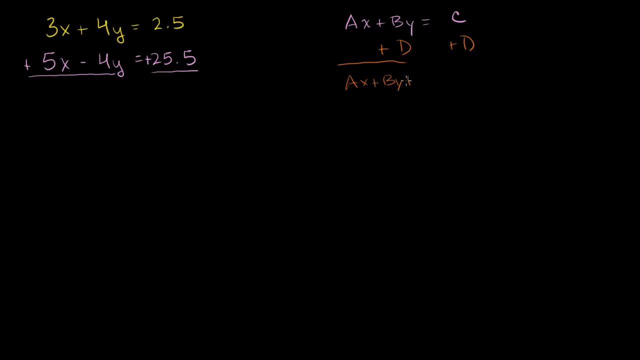 You would get ax plus by plus d is equal to c plus d And we've seen that multiple, multiple times. You could add anything you do to one side of the equation you have to do to the other side, But you're saying, hey, Sal, wait. 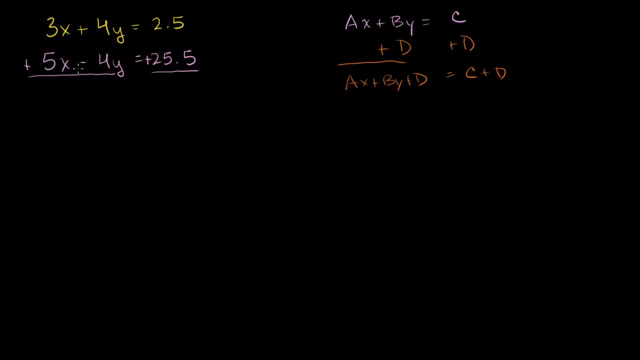 You know, on the left-hand side you're adding 5x minus 4y to the equation. On the right-hand side, you're adding 25.5 to the equation. Aren't you adding two different things to both sides of the equation? 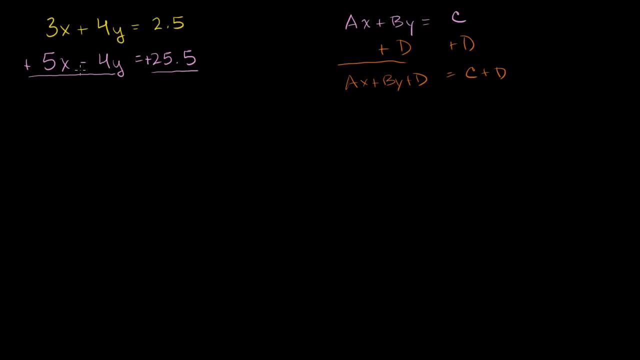 Yes And my answer would be no. We know that 5x minus 4y is 25.5.. And this quantity are the same. They are both 25.5.. This second equation is telling me that explicitly, So I could add this to the left-hand side. 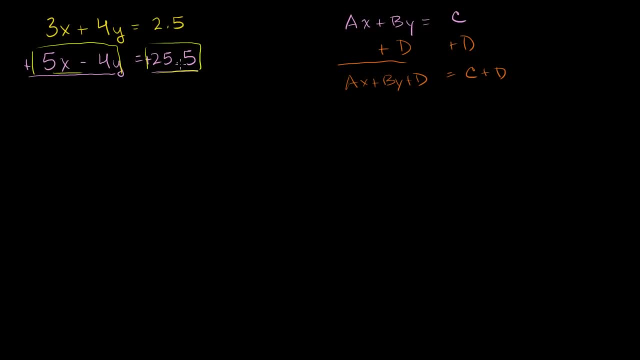 I'm essentially adding 25.5 to it, And I could add 25.5 to the right-hand side. So let's do that. If we were to add the left-hand side, 3x plus 5x is 8x. 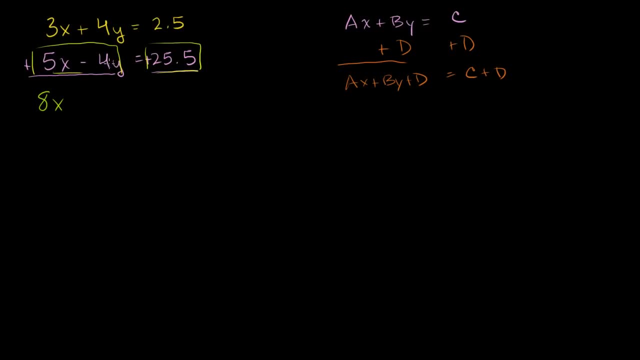 And then what is 4y minus 4y? And this was the whole point I saw. when I looked at these two equations I said, oh, I have a 4y, I have a negative 4y, If you just add these two together. 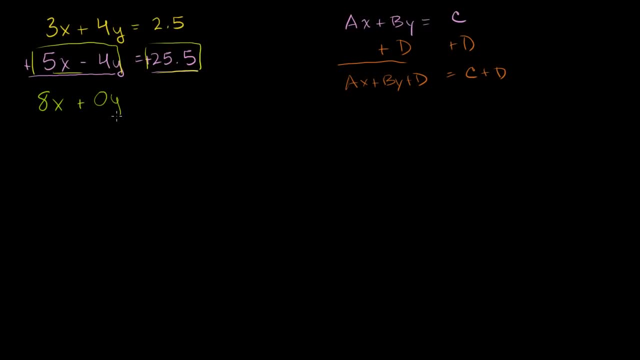 they are going to cancel out. They're going to be plus 0y or that whole term is just going to go away And that's going to be equal to 2.5 plus 25.5 is 28.. So you divide both sides, so you get: 8x is 0.5.. 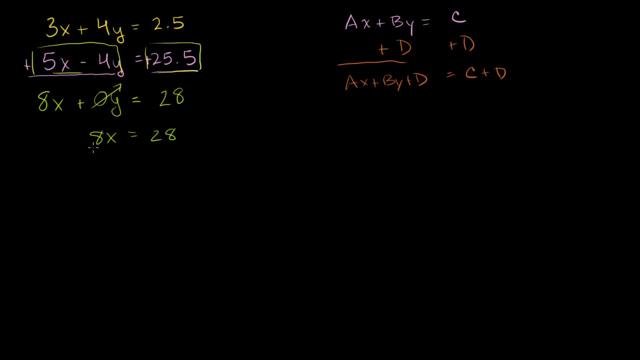 Is equal to 28.. And you divide both sides by 8. And we get: divide both sides, you get: x is equal to 28 over 8.. Or you divide the numerator and the denominator by 4. That's equal to 7 over 2.. 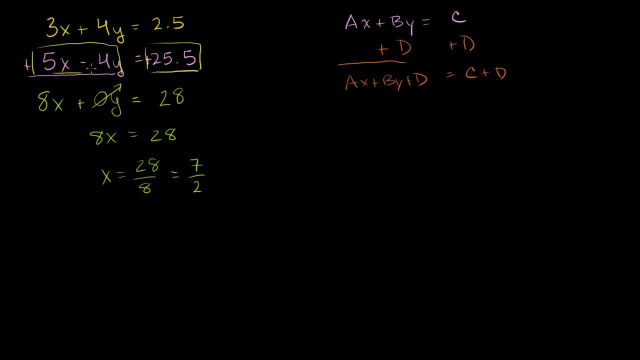 That's our x value. Now we want to solve for our y value And we could substitute this back into either of these two equations. Let's use the top one. You could do it with the bottom one. You could do it with the bottom one as well. 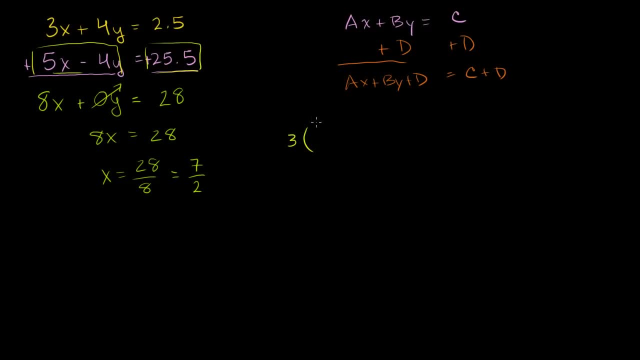 So we know that 3 times x, 3 times 7 over 2, I'm just substituting the x value we figured out into this top equation- 3 times 7 over 2 plus 4y is equal to 2.5. 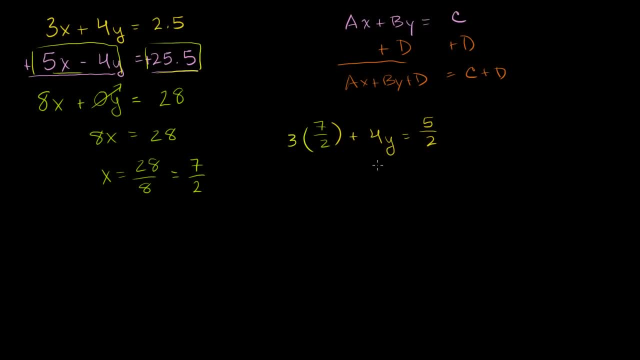 Let me just write that as 5 halves, We're going to stay in the fraction world, So this is going to be 21 over 2 plus 4y is equal to 5 halves Subtract 21 over 2 from both sides. 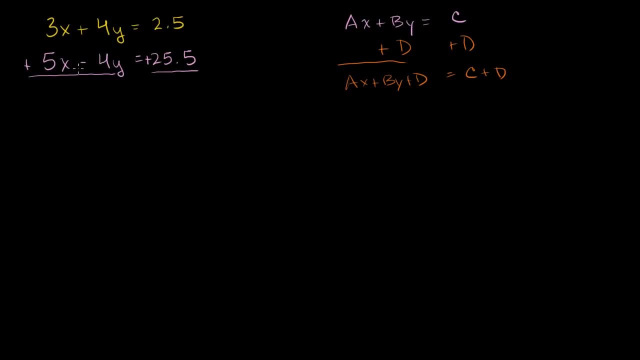 You know, on the left-hand side you're adding 5x minus 4y to the equation. On the right-hand side, you're adding 25.5 to the equation. Aren't you adding two different things to both sides of the equation? 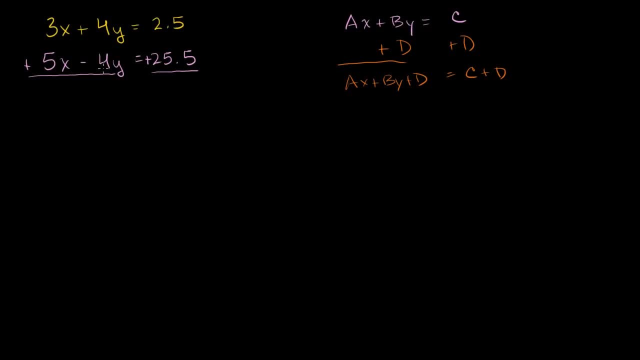 And my answer would be no. We know that 5x minus 4y is 25.5.. And this quantity are the same. They are both 25.5.. This second equation is telling me that explicitly, So I could add this to the left-hand side. 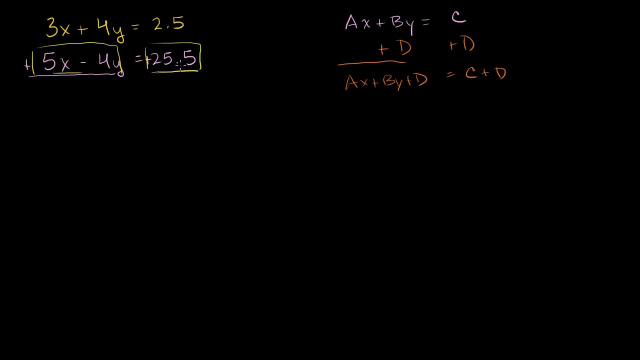 I'm essentially adding 25.5 to it, And I could add 25.5 to the right-hand side. So let's do that. If we were to add the left-hand side, 3x plus 5x is 8x. 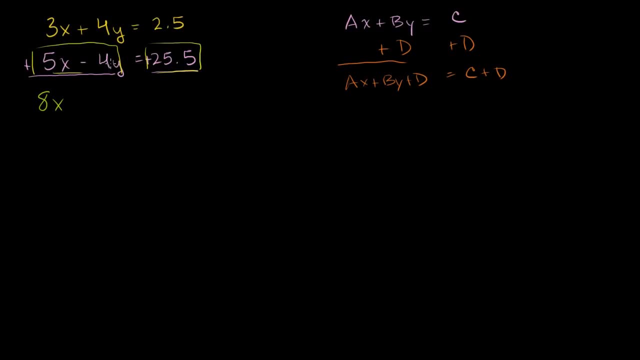 And then, what is 4y minus 4y? And this was the whole point. I saw, you know, when I looked at these two equations, I said, oh, I have a 4y, I have a negative 4y. 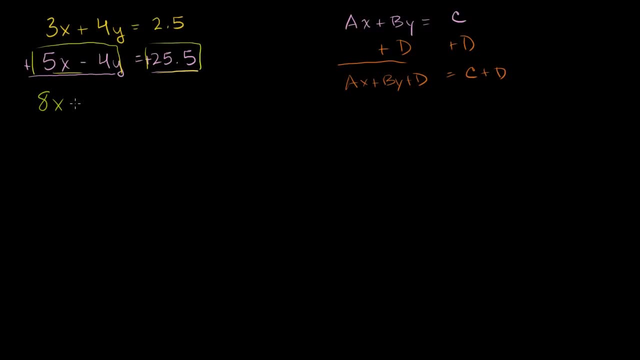 If you just add these two together, they are going to cancel out. They're going to be plus 0y Or that whole term is just going to go away, And that's going to be equal to 2.5 plus 25.5 is 28.. 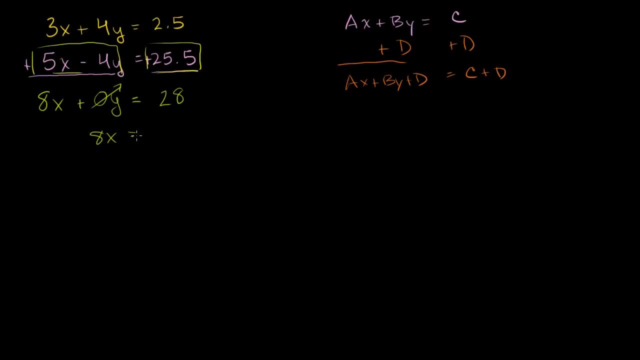 So you divide both sides, So you get: 8x is equal to 28.. And you divide both sides by 8. And we get: divide both sides, You get x is equal to 28 over 8.. Or you divide the numerator and the denominator by 4.. 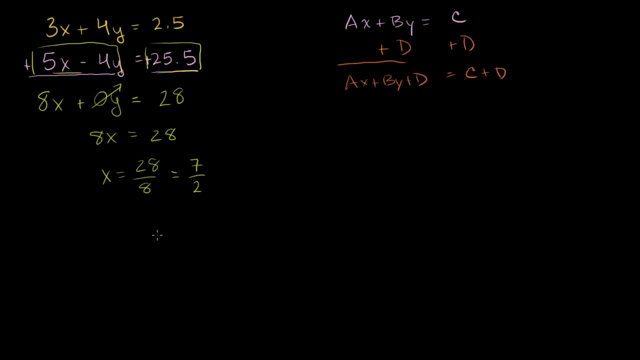 That's equal to 7 over 2.. That's our x value. Now we want to solve for our y value And we could substitute this back into either Either Of these two equations. Let's use the top one. You could do it with the bottom one as well. 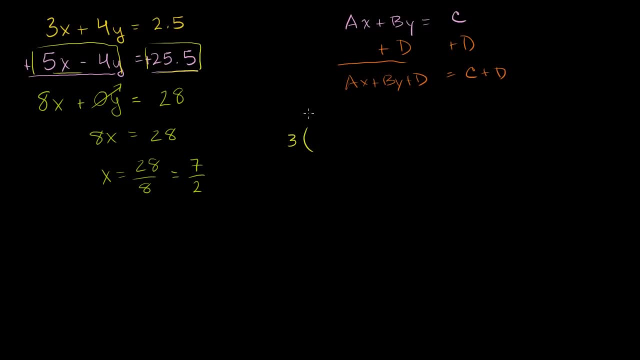 So we know that 3 times x, 3 times 7 over 2, I'm just substituting the x value we figured out into this top equation- 3 times 7 over 2 plus 4y is equal to 2.5. 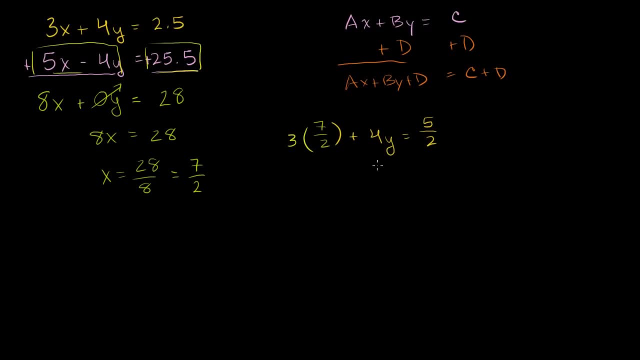 Let me just write that as 5 halves. We're going to stay in the fraction world, So this is going to be 21 over 2.. Plus 4y is equal to 5 halves Subtract 21 over 2 from both sides. 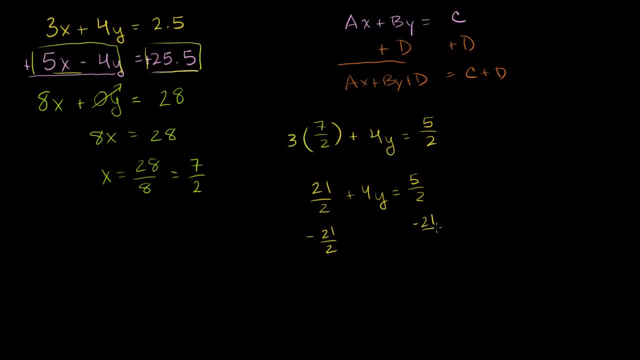 So minus 21 over 2, minus 21 over 2.. The left-hand side- you're just left with a 4y because these two guys cancel out- is equal to: this is 5 minus 21 over 2.. 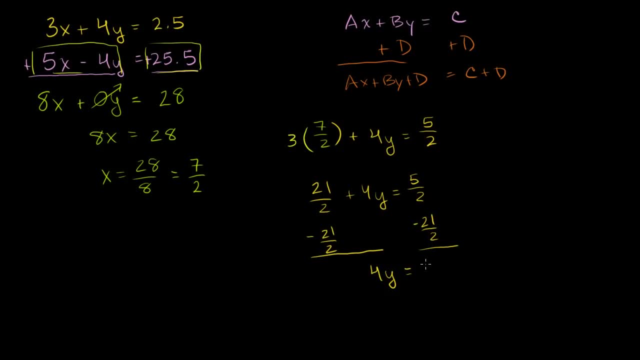 That's negative 16 over 2.. So that's negative 16 over 2, which is the same thing. Well, I'll write it out: That's negative 16 over 2.. Or we could write that I'll continue up here. 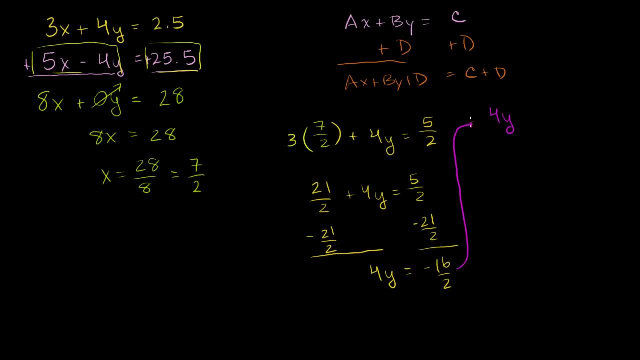 4y- I'm just continuing this train of thought up here- 4y is equal to negative 8.. Divide both sides by 4, and you get y is equal to negative 2. So the solution to this equation is: x is equal to 7 halves. 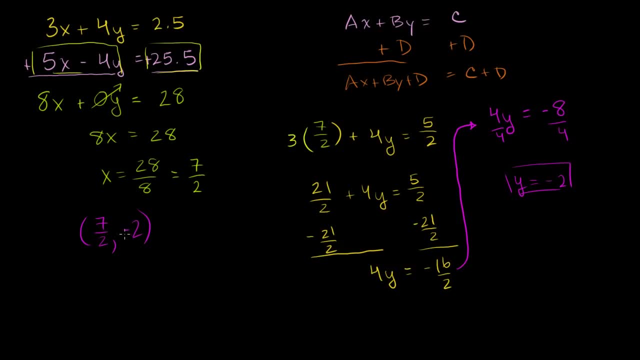 y is equal to negative 2.. This would be the coordinate of their intersection And you could try it out on both of these equations right here. So let's verify that it also satisfies this bottom equation: 5 times 7 halves is 35 over 2, minus 4 times negative 2.. 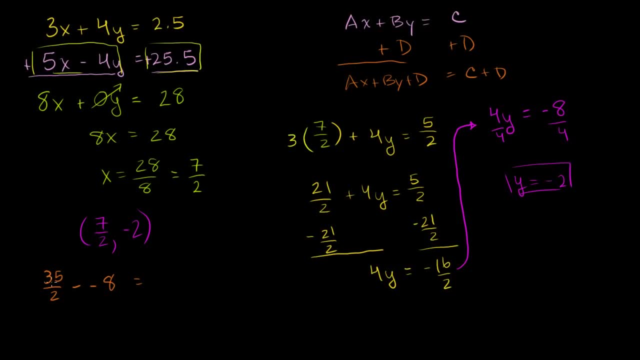 So minus negative 8. That's equivalent to see this is 17.5 plus 8.. This is 17.5,, this is plus 8. And that indeed does equal 25.5.. So this satisfies both equations. 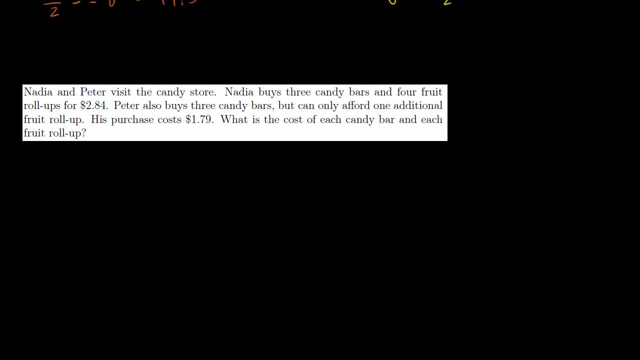 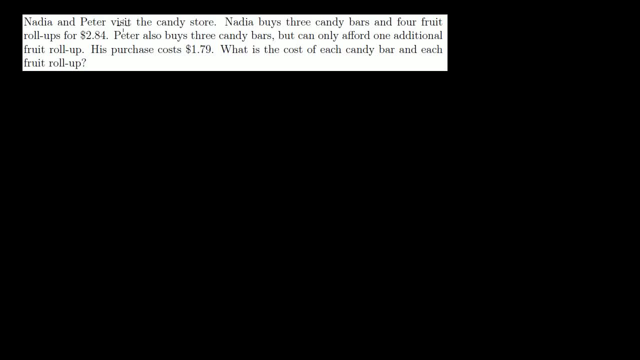 Now let's see if we can use our newly found skills to tackle a word problem, Our newly found skills in elimination. So here it says: Nadia and Peter visit the candy store. Nadia buys three candy bars and four fruit roll-ups for $2.84.. 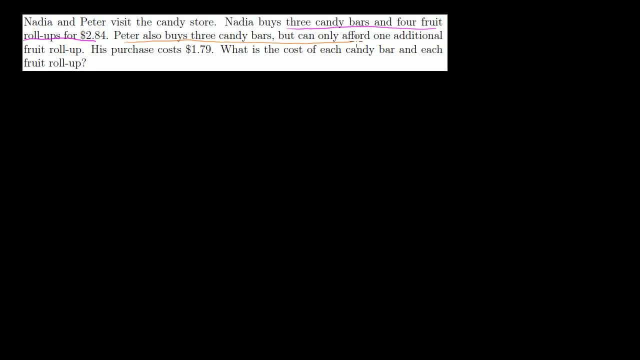 Peter also buys three candy bars but can only afford one additional fruit roll-up. His purchase cost is $1.79.. What is the cost of each candy bar And each fruit roll-up? So let's define some variables. Well, let's just use x and y. 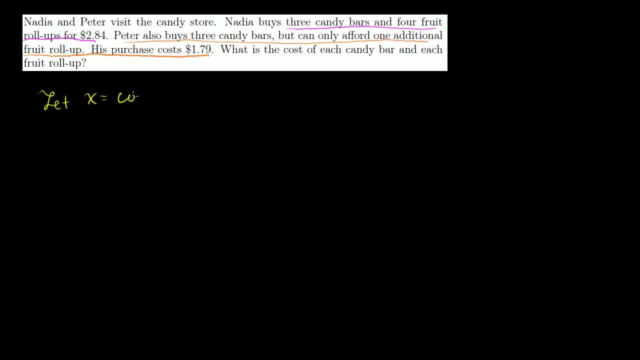 Let's let x equal cost of candy bar. I was going to do a c and a f for fruit roll-up, but I'll just stick with x and y Cost of candy bar And let y equal the cost of a fruit roll-up. 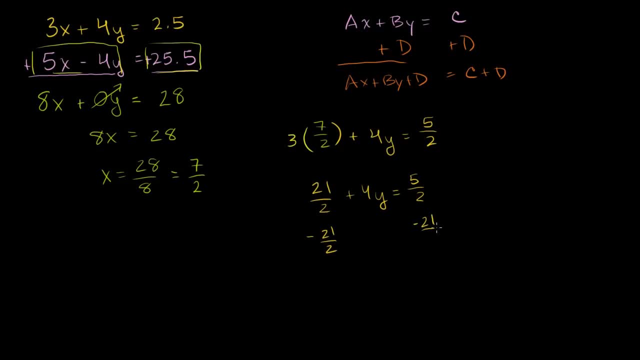 So minus 21 over 2.. Minus 21 over 2.. The left-hand side: you're just left with a 4y Because these two guys cancel out Is equal to: this is 5 minus 21 over 2.. 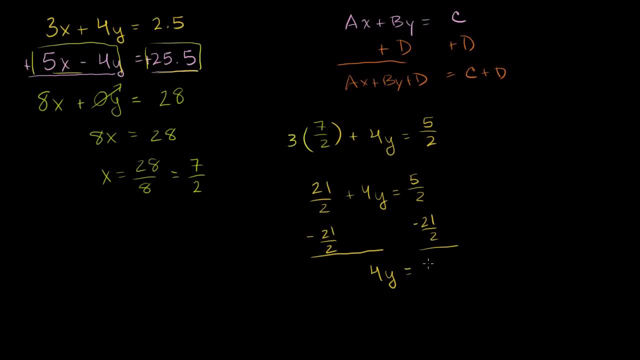 That's negative 16 over 2.. So that's negative 16 over 2.. Which is the same thing. Well, I'll write it out: Negative 16 over 2.. Or we could write that: let's continue up here. 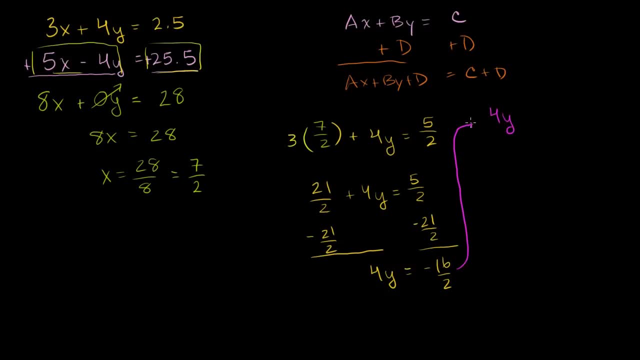 4y- I'm just continuing this train of thought up here- 4y is equal to negative 8. Divide both sides by 4. And you get y is equal to negative 2. So the solution to this equation is: x is equal to 7. 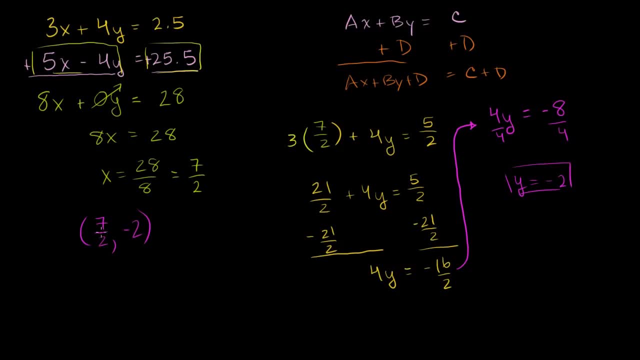 halves y is equal to negative 2.. This would be the coordinate of their intersection And you could try it out on both of these equations right here. So let's verify that. it also satisfies this bottom equation: 5 times 7 halves is 35 over 2.. 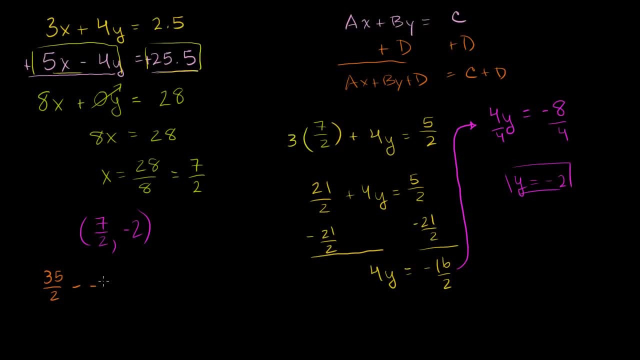 Minus 4 times negative 2. So minus negative 8. That's equivalent to see. this is 17.5 plus 8.. Right, this is 17.5.. This is plus 8. And that indeed does equal 25.5.. 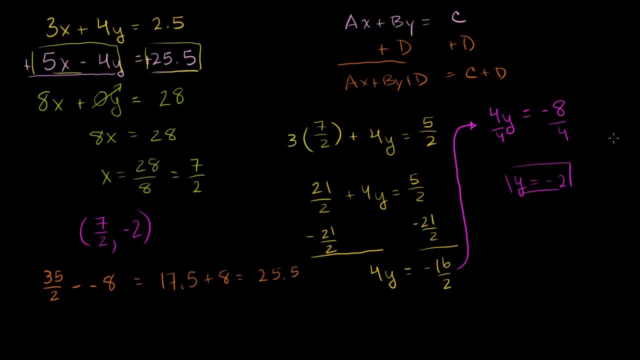 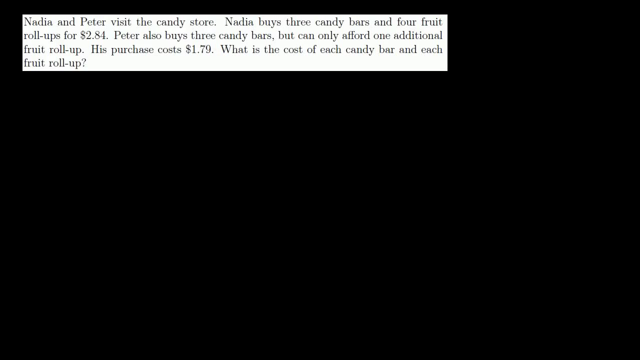 So this satisfies both equations. Now let's see if we can use our newly found skills to tackle a word problem, Our newly found skills in elimination. So here it says: Nadia and Peter visit the candy store. Nadia buys three candy bars and four fruit roll-ups for $2.84.. 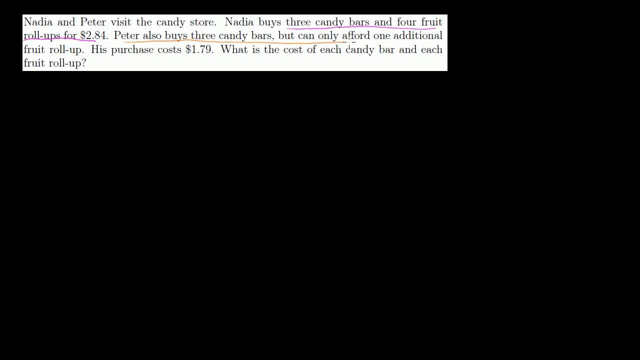 Peter also buys three candy bars but can only afford one additional fruit roll-up. His purchase cost is $2.85.. $2.79.. What is the cost of each candy bar and each fruit roll-up? So let's define some variables. 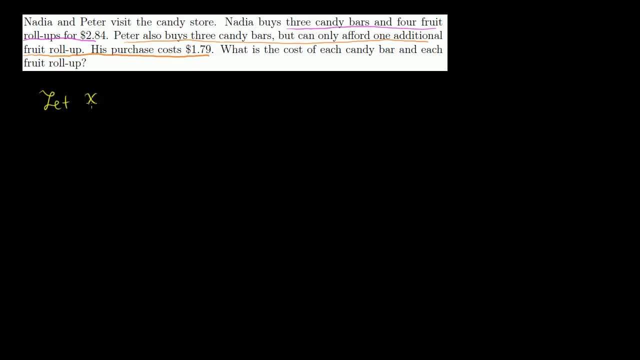 Well, let's just use x and y. Let's let x equal cost of candy bar. I was going to do a c and a f for fruit roll-up, but I'll just stick with x and y Cost of candy bar And let y equal the cost of a fruit roll-up. 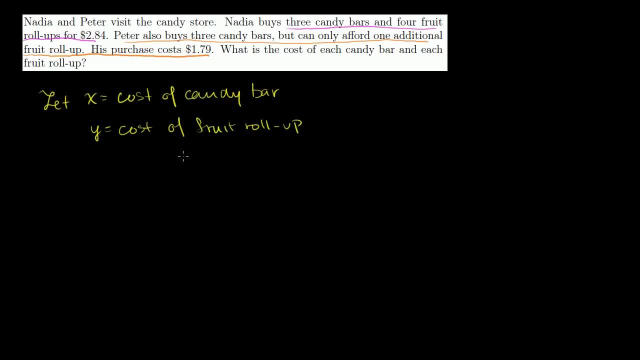 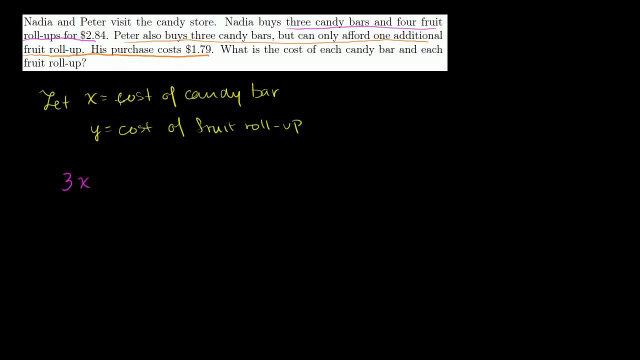 Three times the cost of a candy bar and four fruit roll-ups, Plus 4 times y the cost of a fruit roll-up. This is how much Nadia spends: Three candy bars, four fruit roll-ups And it's going to cost $2.84.. 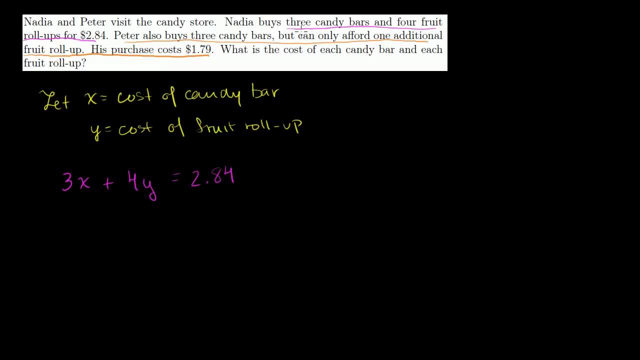 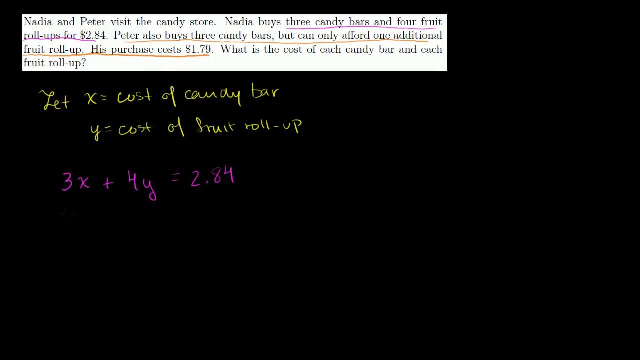 The second statement. Peter also buys three candy bars. Peter also buys three candy bars but can only afford one additional fruit roll-up. So plus one additional fruit roll-up, His purchase cost is equal to $1.79.. What is the cost of each candy bar and each fruit roll-up? 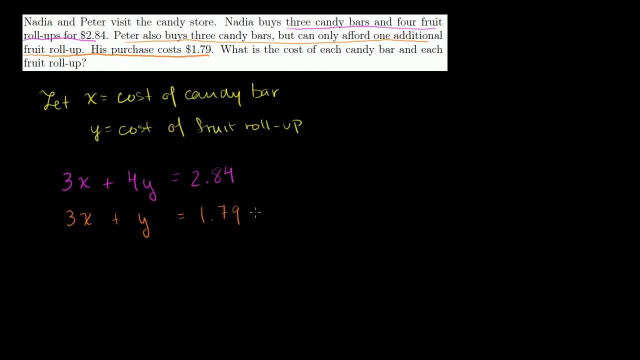 And we're going to solve this using elimination. You could solve this using any of the techniques we've seen so far: Substitution, elimination, even graphing, Although it's kind of hard to eyeball things with the graphing. So how can we do this? 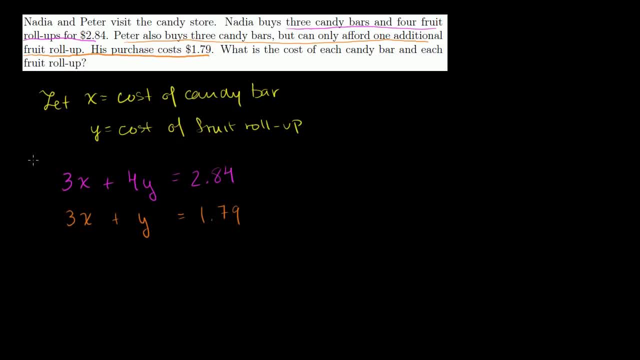 Remember, with elimination you're going to add. Let's focus on this top equation right here. Is there something we can add to both sides of this equation that will help us eliminate one of the variables? Or let me put it this way: 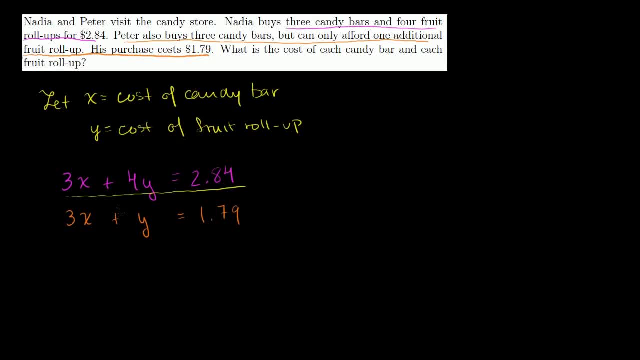 Is there something we could add or subtract to both sides of this equation that will help us eliminate one of the variables? Well, like in the problem we did a little bit earlier in the video, OK, What if we were to subtract this equation? 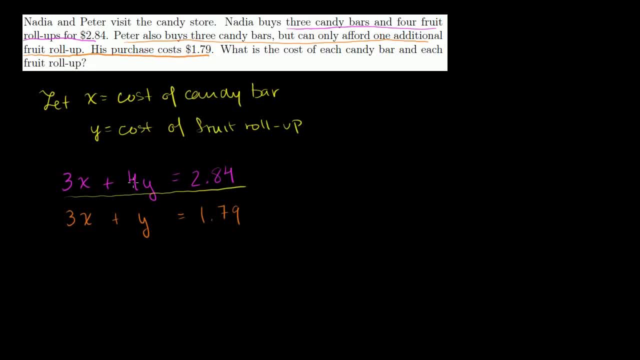 or what if we subtract 3x plus y from 3x plus 4y on the left-hand side and subtract $1.79 from the right-hand side, And remember, by doing that I would be subtracting the same thing from both sides? 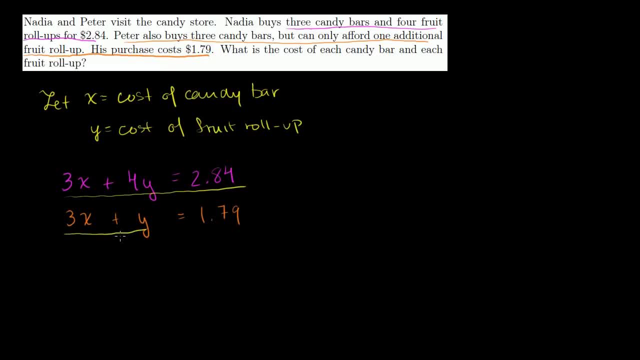 of the equation, This is $1.79.. How do I know? Because it says this is equal to $1.79.. So if we did that, we would be subtracting the same thing from both sides of the equation. So let's subtract 3x plus y from the left-hand side. 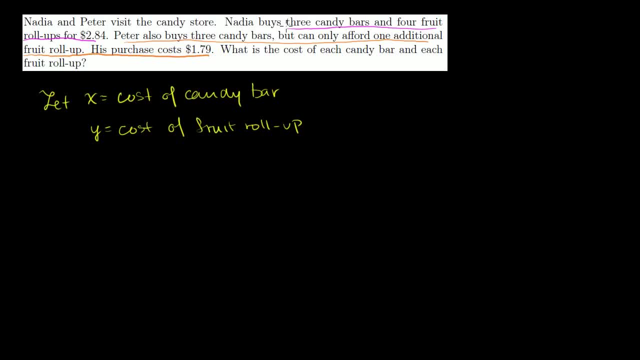 All right. So what is this? This first statement tells us: Nadia buys three candy bars, So the cost of three candy bars is going to be 3x. Three candy bars, Three times the cost of a candy bar and four fruit roll-ups. 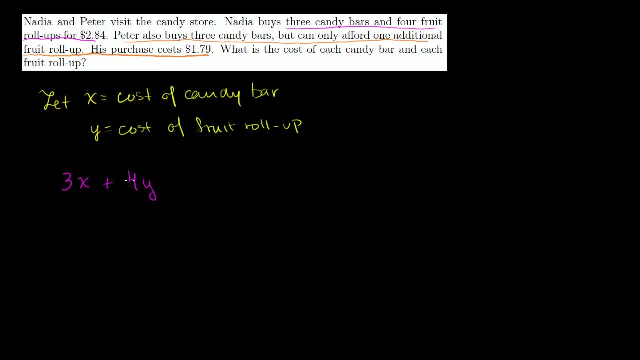 Plus four times y the cost of a fruit roll-up. This is how much Nadia spends: Three candy bars, four fruit roll-ups And it's going to cost $2.84.. That's what this first statement tells us. It translates into that equation. 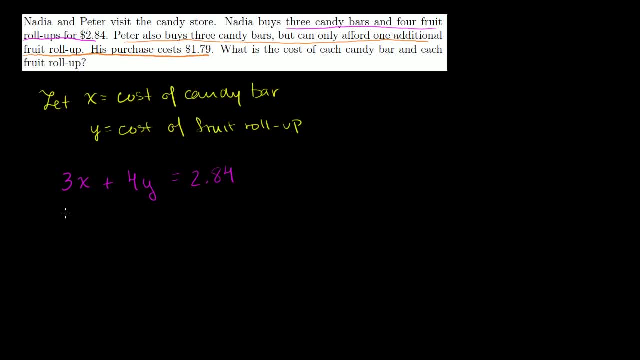 The second statement. Peter also buys three candy bars But can only afford one additional fruit roll-up. So plus one additional fruit roll-up, his purchase cost is equal to $1.79.. What is the cost of each candy bar and each fruit roll-up? 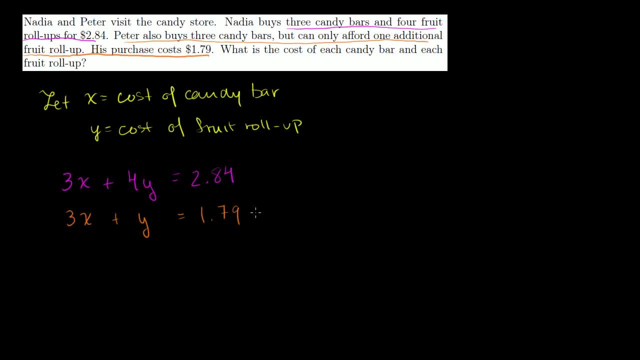 And we're going to solve this using elimination. You could solve this using any of the techniques we've seen so far: Substitution, elimination, even graphing, although it's hard to eyeball things, things with the graphing. So how can we do this? 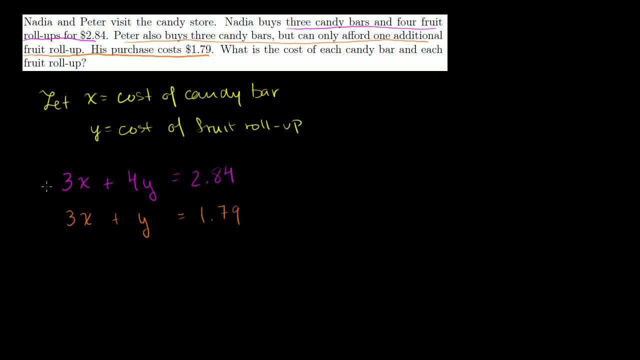 Remember, with elimination you're going to add. let's focus on this top equation right here. Is there something we can add to both sides of this equation that will help us eliminate one of the variables? or let me put it this way: is there something? 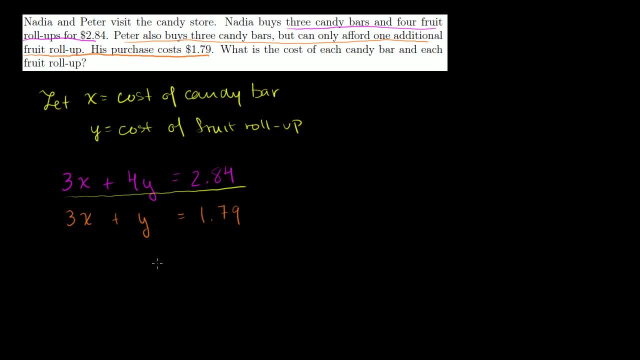 we could add or subtract to both sides of this equation. that will help us eliminate one of the variables. Well, like in the problem we did a little bit earlier in the video, what if we were to subtract this equation? or what if we subtract 3x plus y from 3x plus 4y on the left? 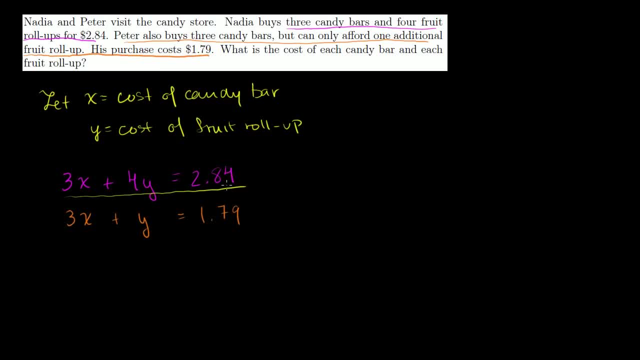 hand side and subtract $1.79 from the right hand side, And remember, by doing that I would be subtracting the same thing from both sides of the equation: This is $1.79.. How do I know? Because it says this is equal to $1.79. 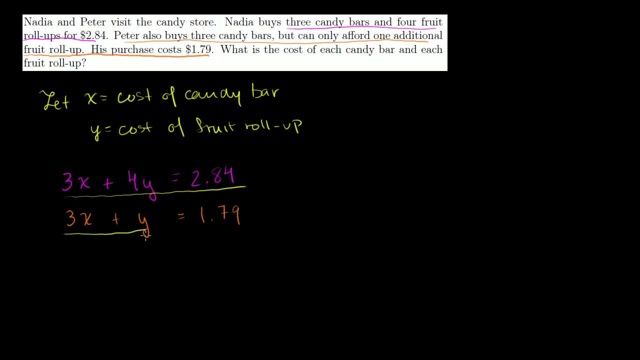 So if we did that, we would be subtracting the same thing from both sides of the equation. So let's subtract 3x plus y from the left hand side of the equation. so I'm going to subtract it from the left hand side and let me just do this over the right. 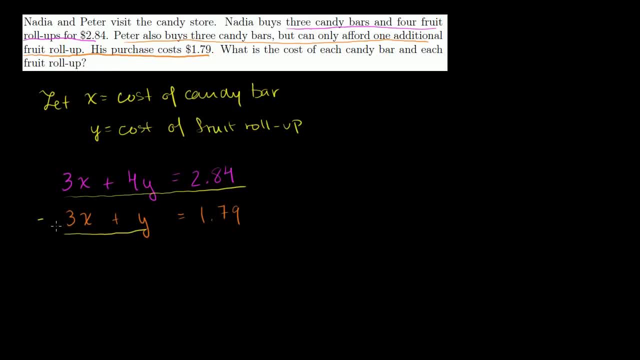 of the equation. So I'm going to subtract it from the left-hand side And let me just do this over the right. If I subtract 3x plus y, that is the same thing as negative 3x minus y, if you just. 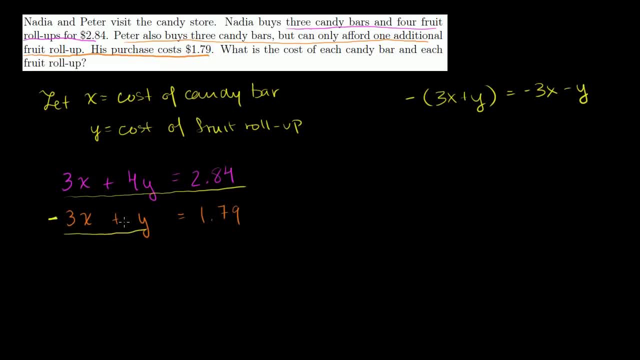 distribute the negative sign, So let's subtract it So you get negative 3x minus y. And maybe I should make it very clear: this is not a plus sign. I'm multiplying. OK, You can imagine I'm multiplying the second equation. 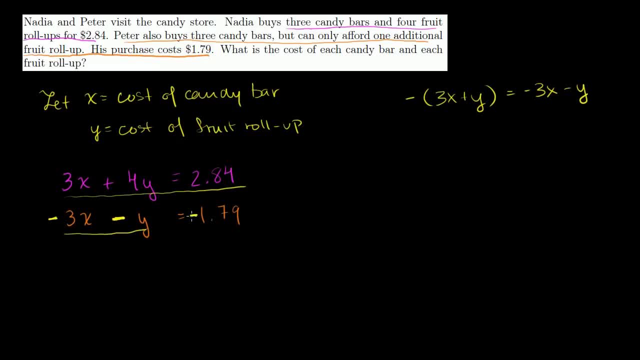 by negative 1 is equal to negative $1.79.. I'm just taking the second equation. You can imagine I'm multiplying it by negative 1.. And now I'm going to add this side, the left-hand side, to the left-hand side of this equation. 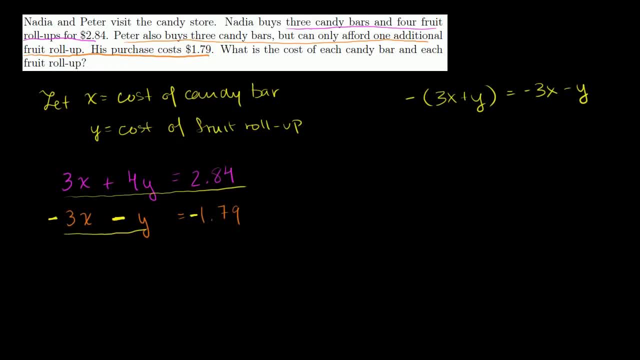 and the right-hand side to the right-hand side of that equation. And what do we get? When you add 3x plus 4y minus 3x minus y, the 3x's cancel out. 3x minus 3x is 0x. 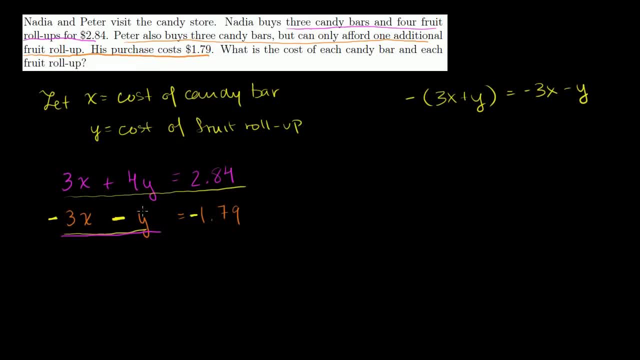 0x. You can even write it down. You get 4y minus y, That is 3y, And that is going to be equal to $2.84 minus $1.79.. What is that? That is like $1.05.. 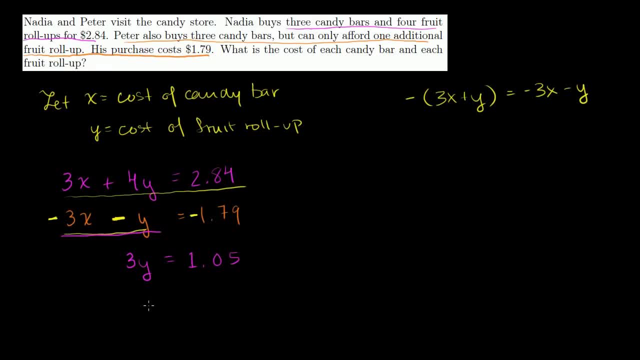 So 3y is equal to $1.05.. Divide both sides by 3.. y is equal to what's $1.05?? Divide both sides by 3.. So 3 goes into $1.05.. It goes into 1, 0 times. 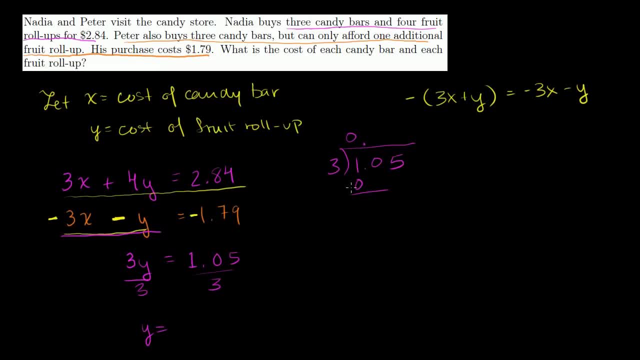 0 times 3 is 0.. 1 minus 0 is 1.. Bring down a 0.. 3 goes into 10. 3 times 3 times 3 is 9.. Subtract 10 minus 9 is 1.. 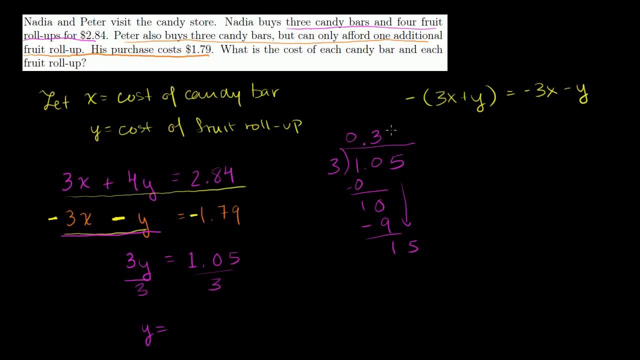 Bring down the 5.. 3 goes into 15. 5 times 5 times 3 is 15.. Subtract: We have no remainder. So y is equal to $0.35.. So the cost of a fruit roll-up is $0.35.. 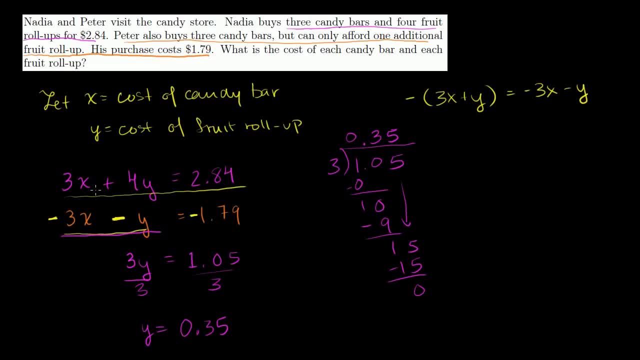 Now we can substitute back into either of these equations to figure out the cost of a candy bar. So let's use this bottom equation right here, Which was originally, if you remember, before I multiplied it by negative 1, it was 3x plus y is equal to $1.79.. 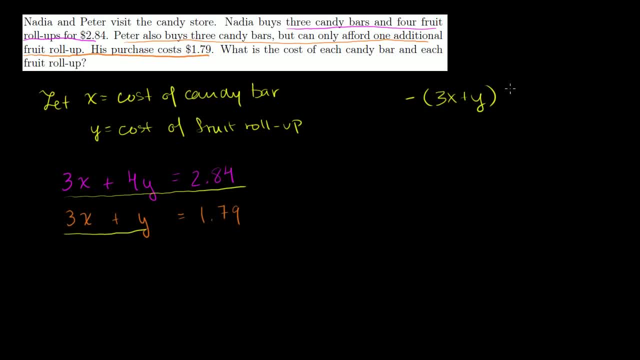 If I subtract 3x plus y, that is the same thing as negative 3x minus y if you just distribute the negative sign. So let's subtract it so you get negative 3x minus y. and maybe I should make it very clear this is not a plus sign. 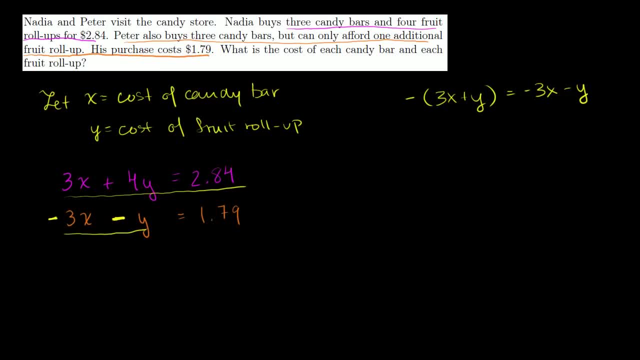 I'm multiplying. You can imagine I'm multiplying the second equation by negative 1, is equal to negative $1.79.. I'm just taking the second equation. You can imagine I'm multiplying it by negative 1,. and now I'm. 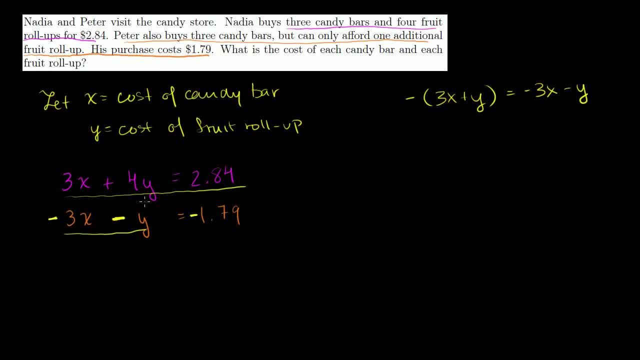 going to add this side, the left hand side, to the left hand side of this equation and the right hand side to the right hand side of that equation. And what do we get? When you add 3x plus 4y minus 3x minus y, the 3x's cancel out. 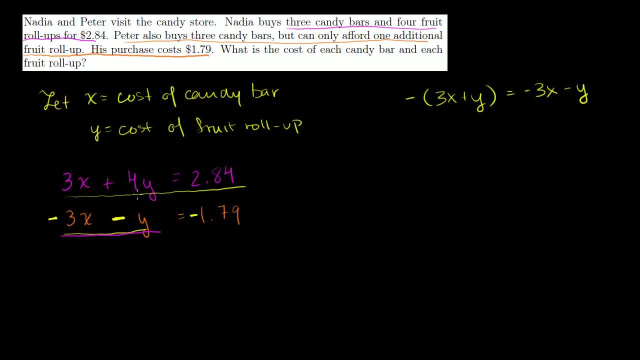 3x minus 3x is 0x. I want to be clear. I didn't even write it down. You get 4y minus y, that is 3y, And that is going to be equal to $2.84 minus $1.79.. 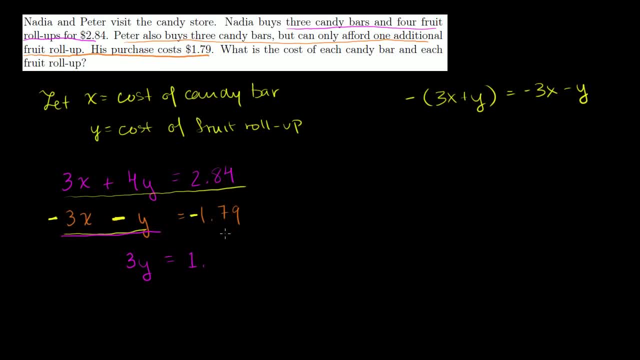 What is that? That's $1.05.. So 3y is equal to $1.05.. Divide both sides by 3.. y is equal to what's $1.05? 5 divided by 3.. So 3 goes into $1.05.. 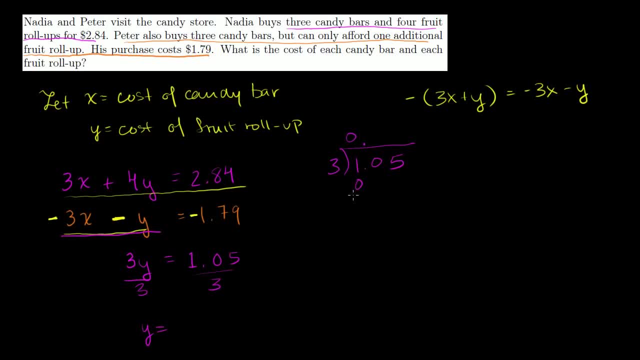 It goes into 1: 0 times 0 times 3 is 0.. 1 minus 0 is 1.. Bring down a 0.. 3 goes into 10. 3 times 3 times 3 is 9.. 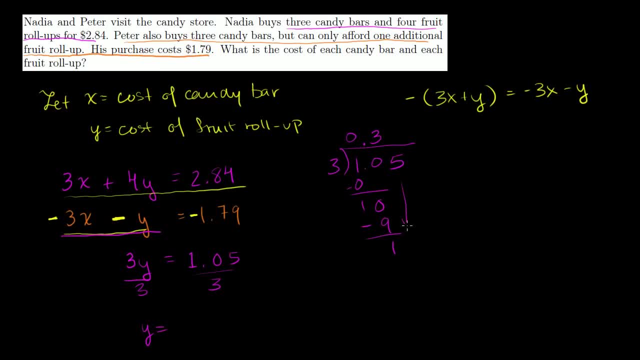 Subtract: 10 minus 9 is 1.. Bring down the 5. 3 goes into 15. 5 times 5 times 3 is 15.. Subtract: We have no remainder, So y is equal to $0.35.. 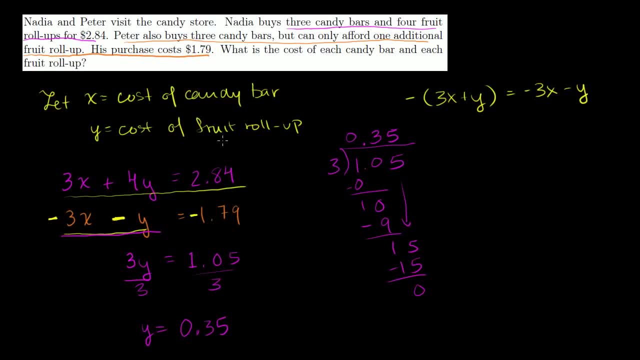 So the cost of a fruit roll-up is $0.35.. Now we can substitute back into either of these equations to figure out the cost of a candy bar. So let's use this bottom equation right here, Which was originally, if you remember, before I multiplied. 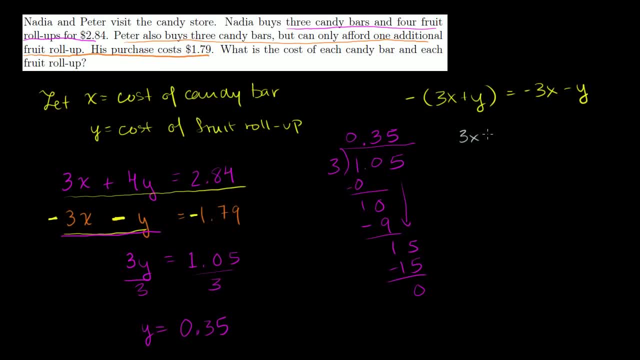 it by negative 1, it was 3x plus y- is equal to $1.79.. So that means that 3x plus the cost of a fruit roll-up- 0.35, is equal to $1.79.. If we subtract 0.35 from both sides, what do we get? 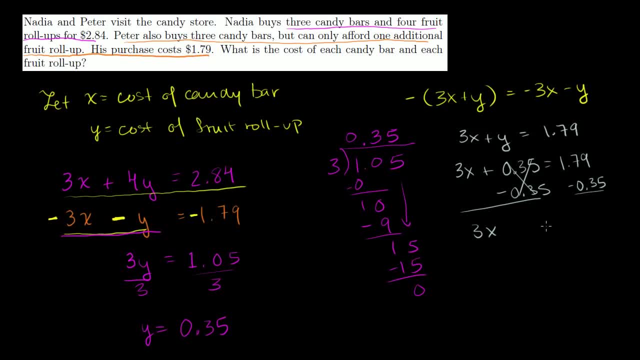 The left-hand side, you're just left with the 3x. These cancel out Is equal to. let's see, this is $1.79 minus 35.. That's $1.44. $1.44. $1.44.. 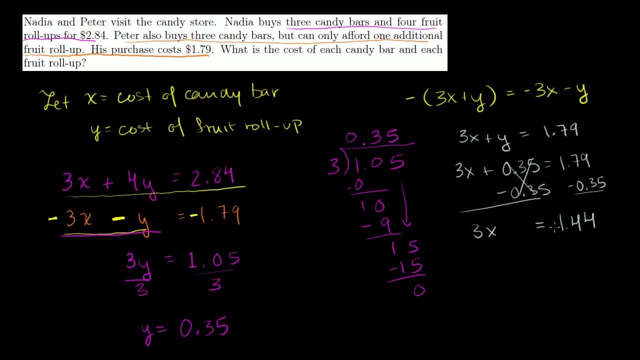 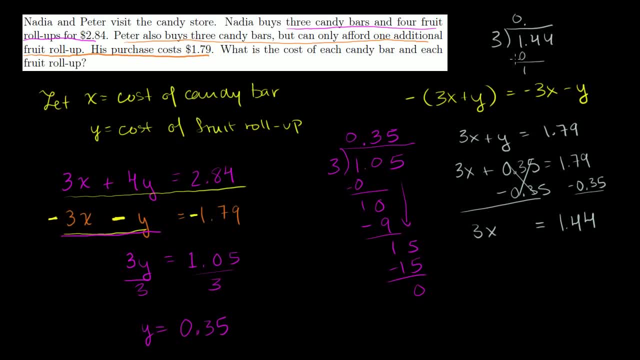 1 times 3 is 0.. Bring down the 1, or subtract Bring down the 4.. 3 goes into 14, 4 times 4 times 3 is 12.. I'm making this messy: 14 minus 12 is 2.. 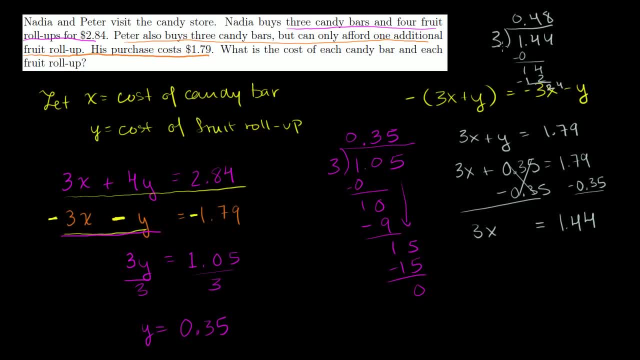 Bring down the 4.. 3 goes into 24.. 8 times 8 times 3 is 24.. No remainder, So x is equal to 0.48.. So there you have it. We figured out using elimination that the cost of 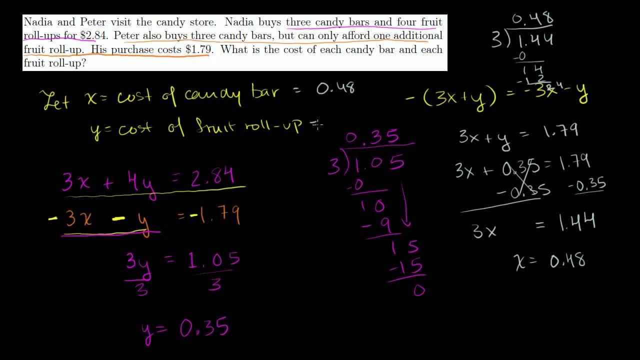 a candy bar is equal to $0.48, and that the cost of a fruit roll-up is equal to $0.35.. 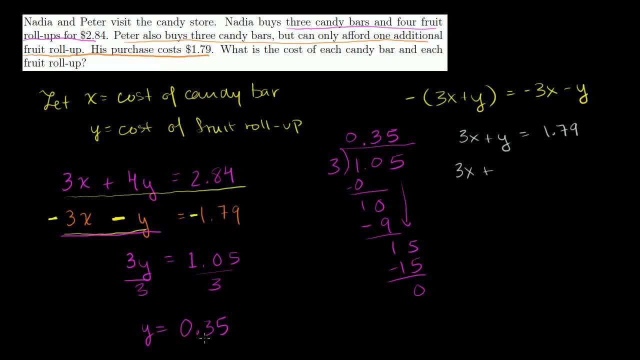 3x plus y is equal to $1.79.. So that means that 3x plus the cost of a fruit roll-up- 0.35, is equal to $1.79.. If we subtract 0.35 from both sides, what do we get? 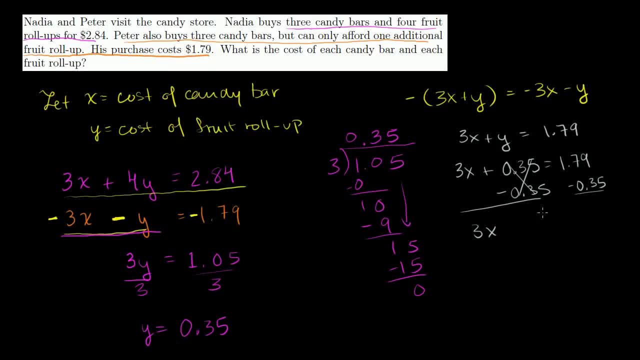 The left-hand side, you're just left with the 3x. These cancel out Is equal to. let's see, this is $1.79 minus 35.. That's $1.44.. And 3 goes into $1.44.. 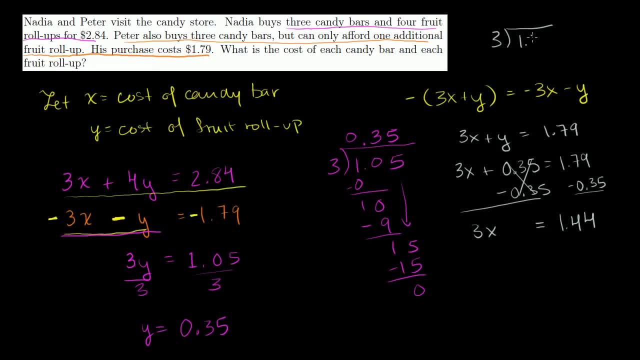 I think it goes well. 3 goes into $1.44.. Goes into 1,, 0 times. 1 times 3 is 0.. Bring down the 1, or subtract bring down the 4.. 3 goes into 14, 4 times. 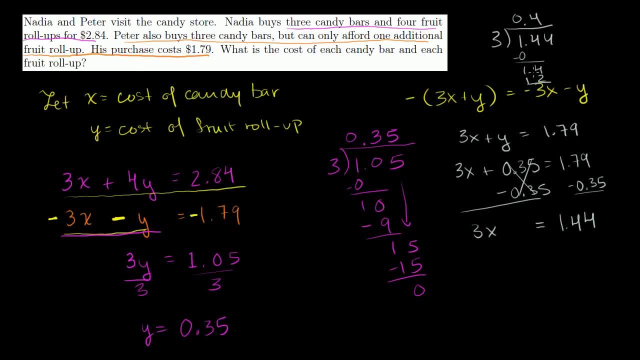 4 times 3 is 12.. I'm making this messy. 12, 14 minus 12 is 2.. Bring down the 4. 3 goes into 24. 8 times 8 times 3 is 24.. 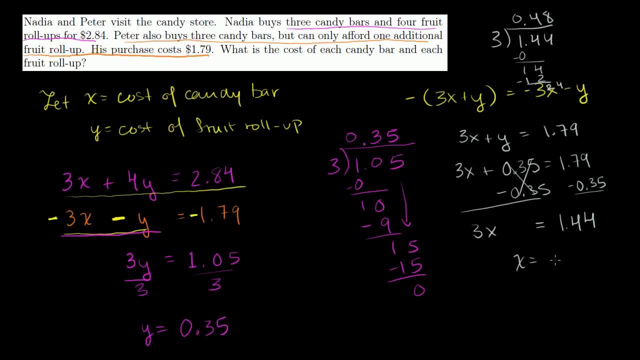 No remainder, So x is equal to 0.48.. So there you have it. We figured out, using elimination, that the cost of a candy bar is equal to $0.48, and that the cost of a fruit roll-up is equal to $0.35.. 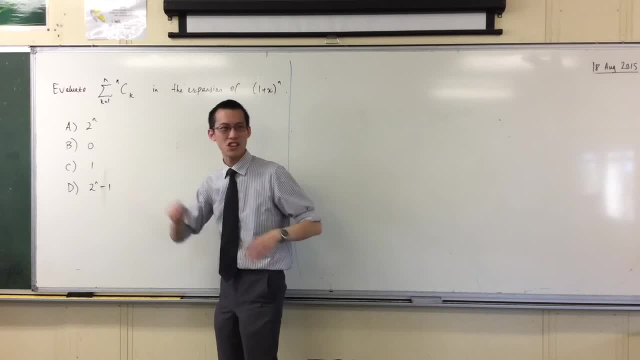 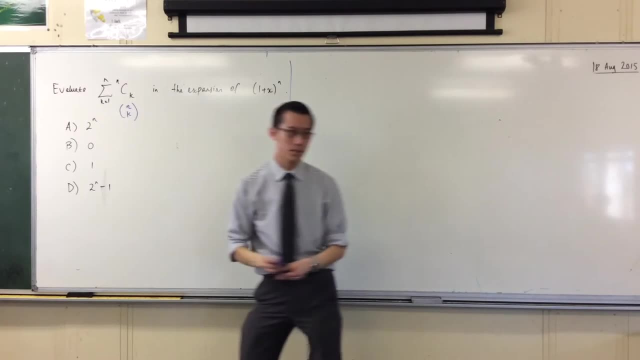 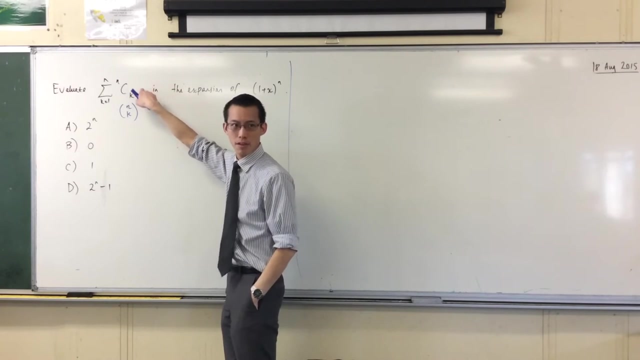 Evaluate this guy here, and you remember this is our ncr notation, which we also write like this: That would be the equivalent, Same deal. Evaluate that from 1 up to n, 1 all the way up to n. So that would be nc1, nc2, nc3, nc4, all the way up to mcn.